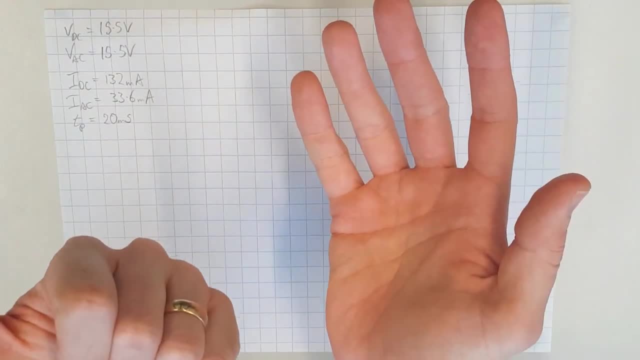 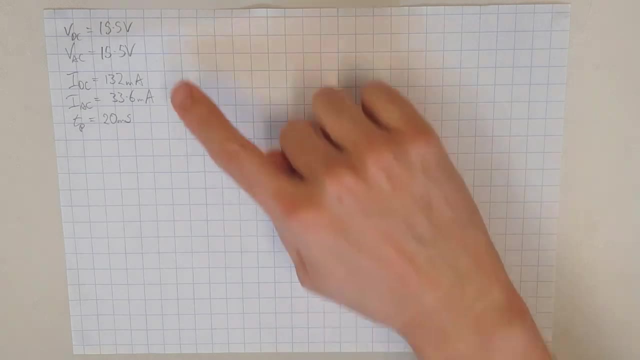 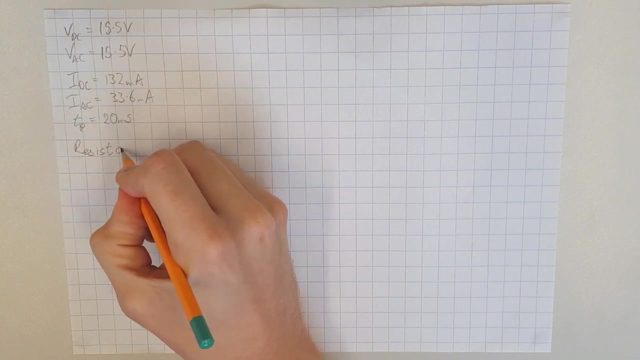 the phase angle and also the capacitance of the capacitor that would be needed to correct the power factor in this circuit. So an awful lot of information can be got from just these few numbers. So first things first, let's figure out how we can calculate the resistance of the coil. Okay. so how can we calculate the resistance of the coil? Well, of course, we know that in a DC circuit, Ohm's law states that I is equal to V over R. Now what we're going to do is we're going to transpose this formula, and in order to do that, we need to do this in a couple of stages. So, first of all, 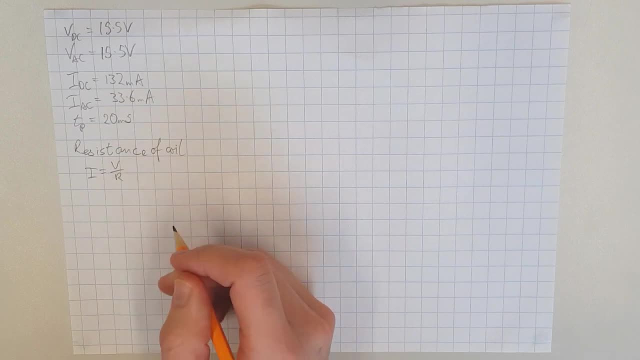 we will multiply both sides by R. so we end up with: if we times both sides by r, this side becomes i times r. and if we times this side by r and then divide it by r, we end up with just v by itself. and then if we want to say, therefore, if i want the r, 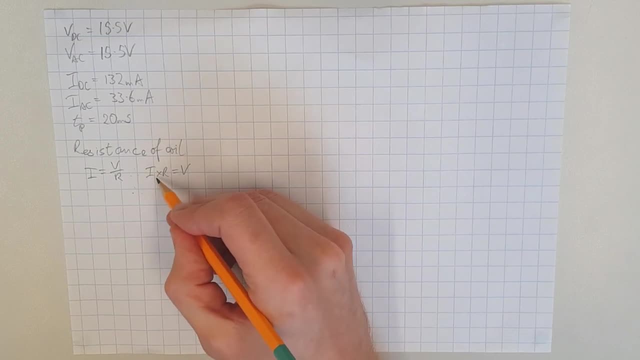 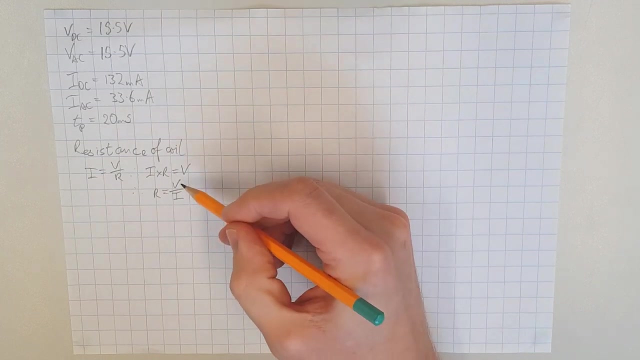 by itself. i need to do the opposite of timesing by i, which is to divide both sides by i, so i end up with: r is equal to v divided by i. now, the only thing that we just need to be a little bit careful about here is we need to make sure that we're using the right voltage and the right current, so 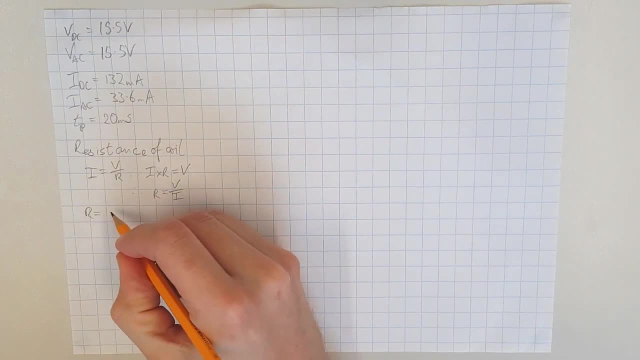 we're going to be a little bit more specific here and we're going to say that r is equal to the dc voltage divided by the dc current, and that's going to tell us what resistance the coil has. so let's just think about that. if i do, the dc voltage, 15.5 volts divided by the dc current. 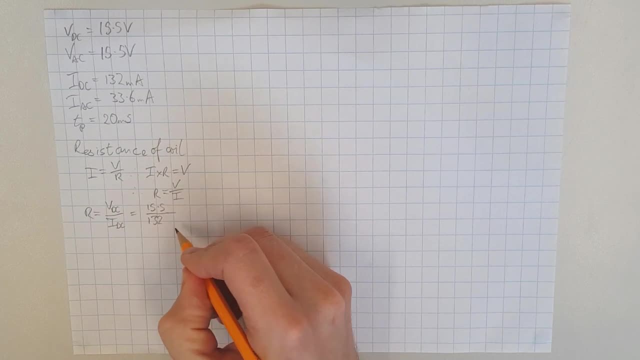 which was 132 milliamps. so there's two ways we could do that. we could put that as 0.132, or we can do it 132 times 10 to the minus three. so we could either just divide this number by a thousand to turn it into amps, or we can tack on the times. 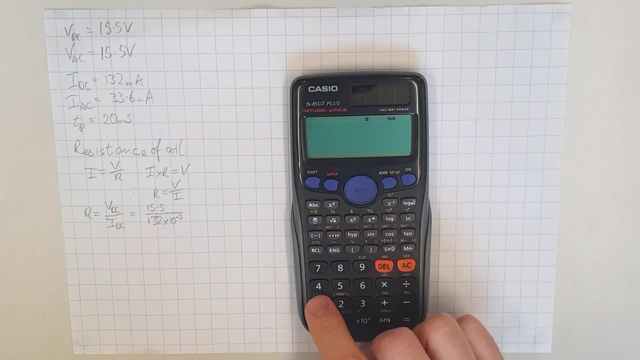 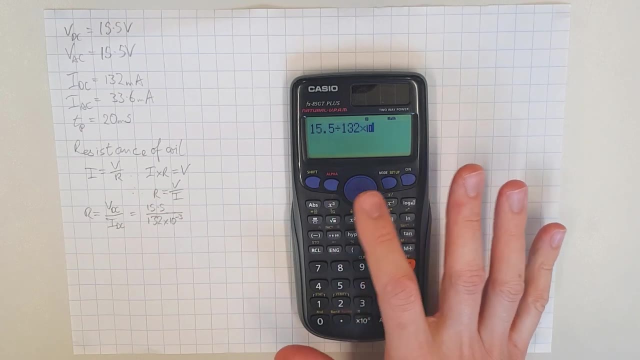 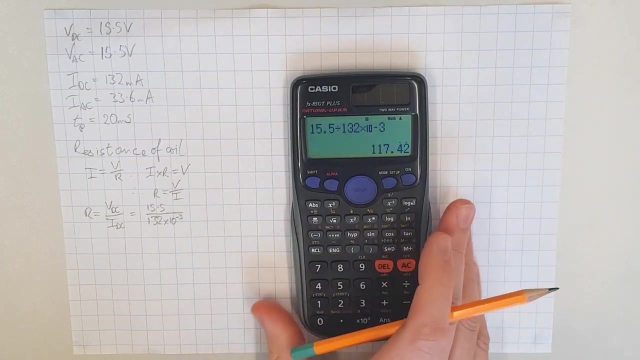 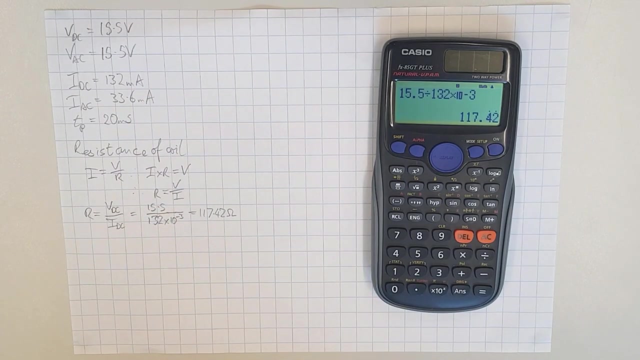 10 to the minus three. so let's put that into our calculator: 15.5 divided by 132 times 10 to the power of minus three, to the power of minus three, which gives us a hundred and seventeen point four, two, and of course this is in ohms. so we've got 117.42 ohms like that, so that coil has a resistance. 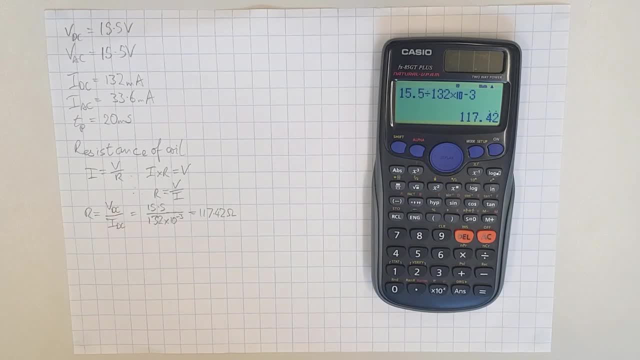 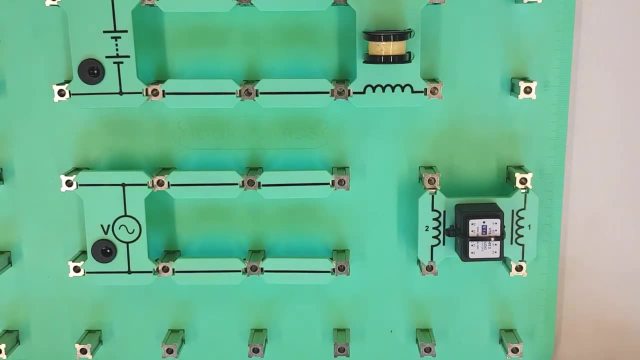 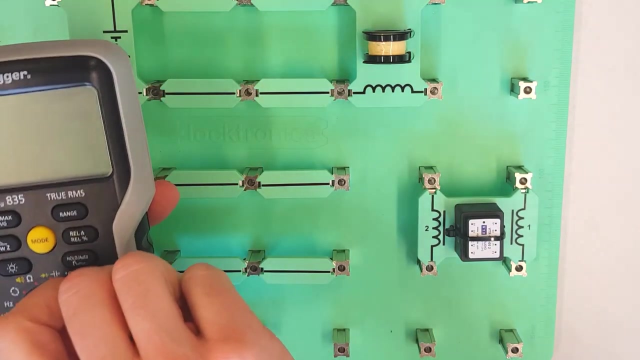 of 117.42 ohms. now we can actually check that by bringing our circuit back in and, as you can see, here we've got the coil that we used in the previous video. so i'm going to set up my mega evo 835 to measure the resistance of the coil. 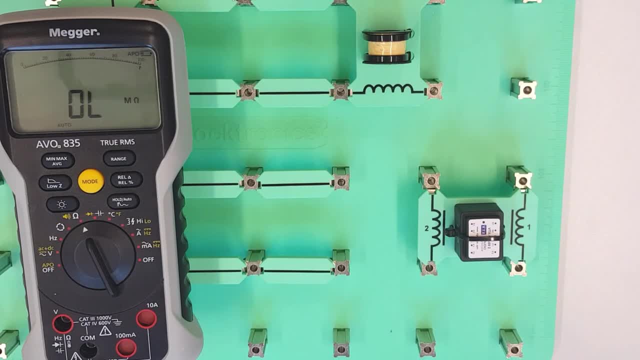 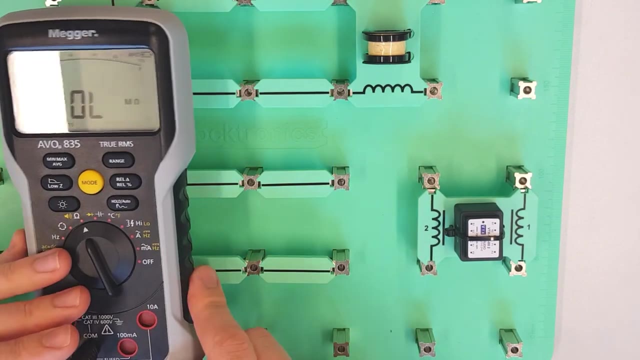 i've just taken the coil out of the circuit, basically, so we can just see that the circuit isn't making any difference to our readings. we're just going to purely measure the resistance of the coil by itself. so there's one lead connected and there's the other lead. 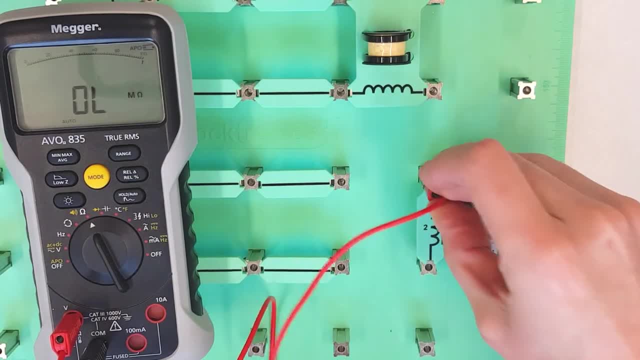 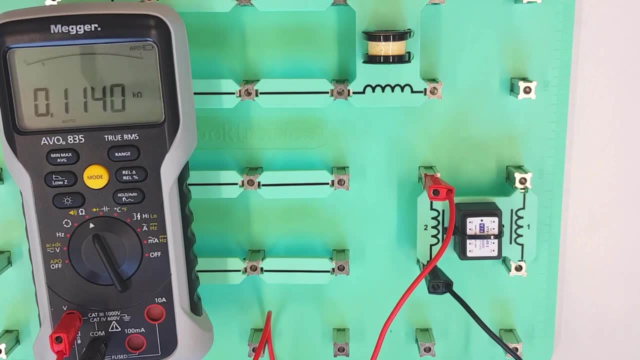 connected and now what we're going to do is we're going to measure the resistance across this coil. so just let it do its auto ranging thing and you can see there we're coming out at about 114 ohms. it says 0.114 because it's measuring in kilo ohms currently. so if we multiply that number by a, 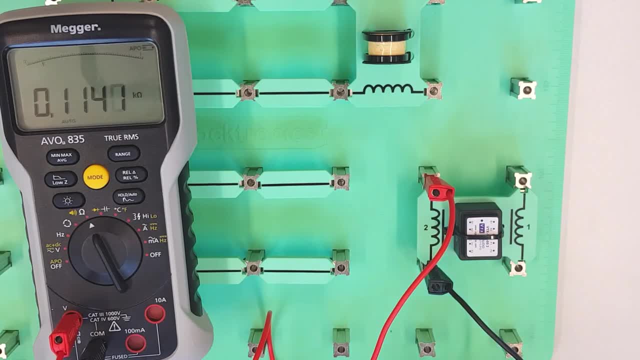 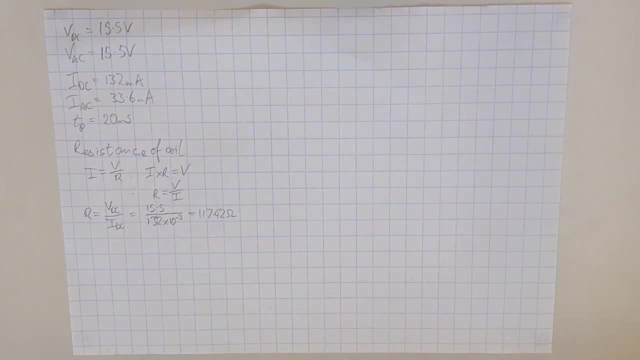 thousand, we end up with 114 ohms, which is very, very close to the value of 117.42 ohms that we calculated that it would be. so we're really happy with that reading and it proves that the maths actually does work. the reason there might be that slight difference there. 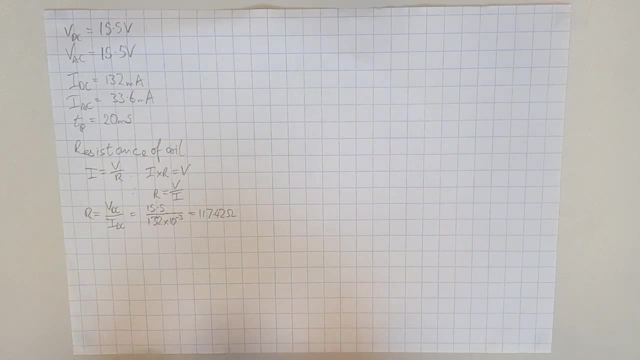 maybe some tolerance within the equipment, maybe a little bit of resistance within the equipment, maybe a little bit of resistance within what we're doing in terms ofRegister LS, the fact that the coil got a little bit warm while we were doing the test, which will affect its resistance, those things might be the reason why this value. 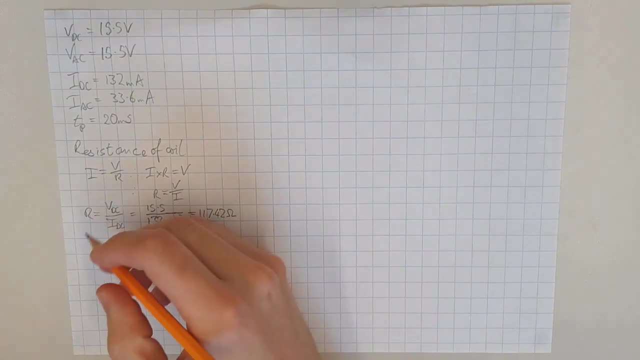 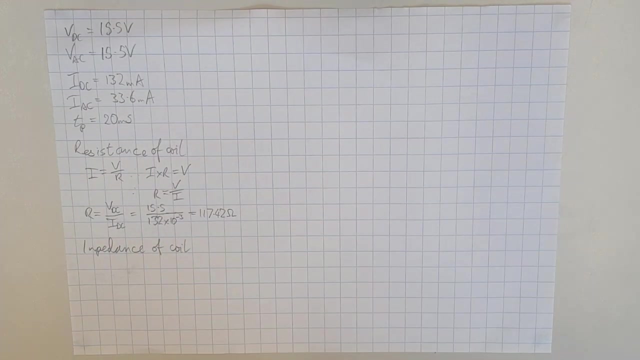 is a little bit higher than we've actually measured there. now the next thing we're going to do is we're going to measure the impedance of the coil. so we'll measure the impedance of the coil. so to calculate the impedance of the coil, we're simply going to reuse I Lane's law, in fact. 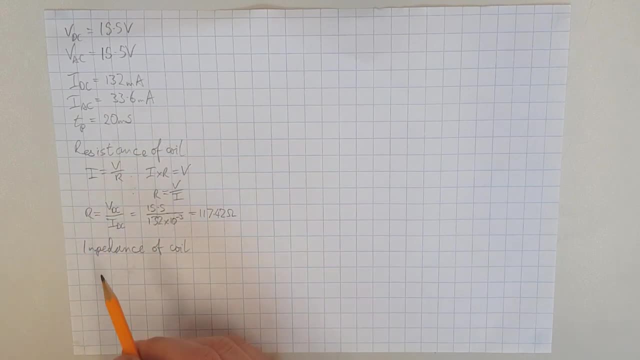 we're going to use this exact same formula that we used last time, but here we were calculating the resistance, which is the opposition to current flow, in a dx ready, like we just did, DC circuit. what we're going to look at in this case is we're going to look at the impedance, so 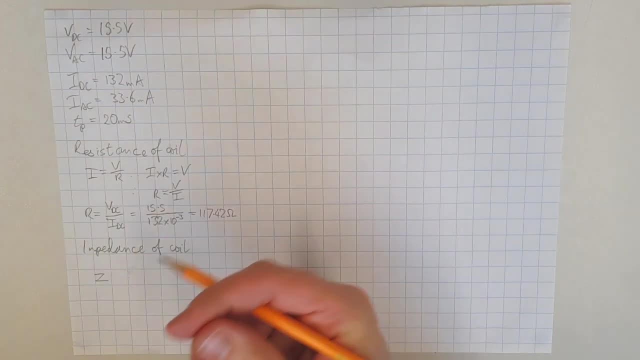 we replace R with Z, because Z is the total opposition to current flow in an AC circuit and we're going to put in here. instead we're going to use VAC, so the AC voltage divided by the AC current. so that's what we're going to use here. so we're going to say that 15.5 divided by 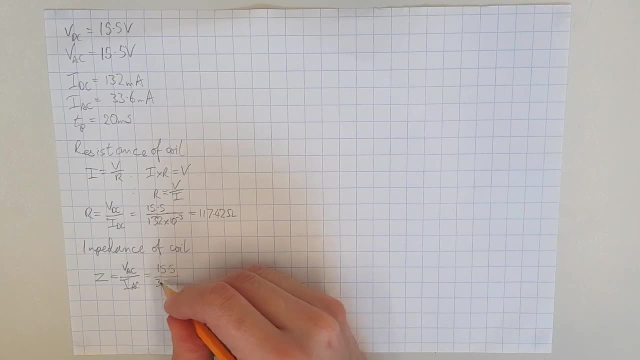 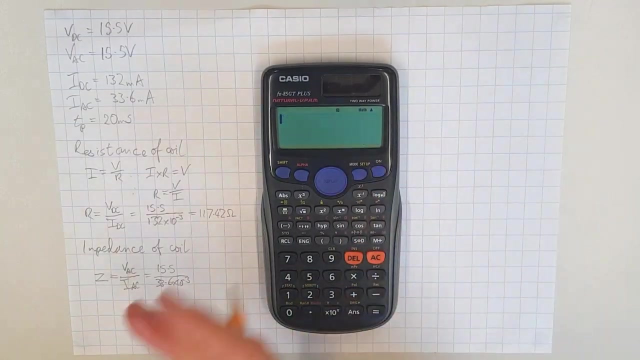 33.6 milliamps. so that's 33.6 times 10 to the minus 3. we're going to figure out what the impedance of the coil is when we connected it to our AC circuit. so 15.5 divided by 33.6. 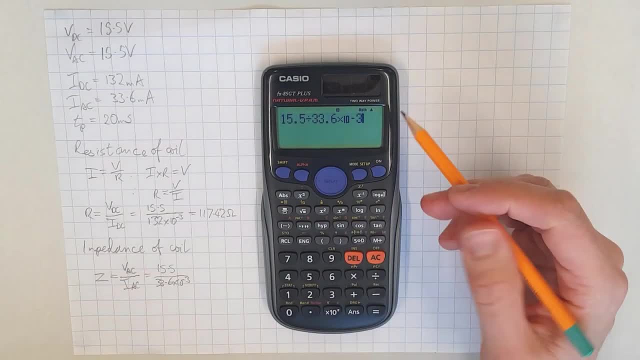 and then we just press the times 10 to the button minus 3. so this number that it puts in after the times 10 is the power that we're raising that 10 to, and again it's exactly the same as dividing this number by a thousand. so we end up with: 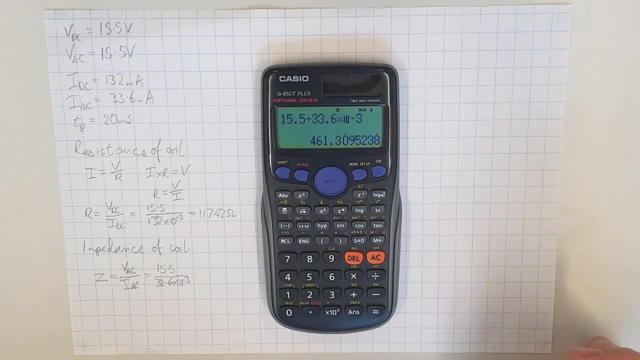 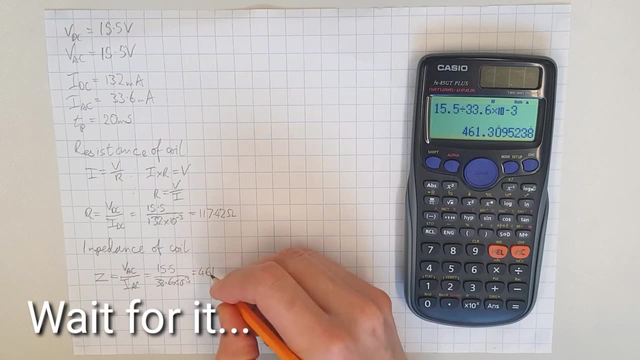 461.3 milliamps. so we'll write that down: 461.3 ohms. it is not milliamps, I beg your pardon, so 461.3 ohms. so what we've noticed is that when we connect this coil up to an AC circuit, the total 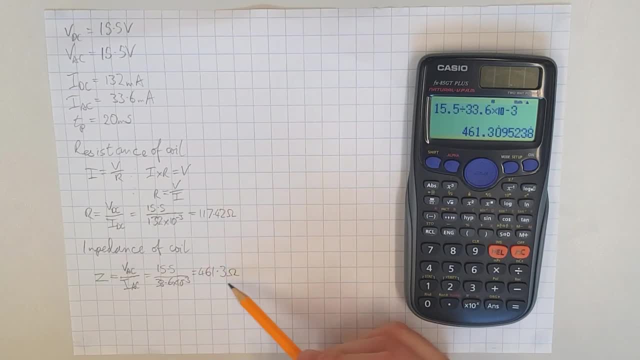 opposition to current flow becomes much larger, quite a significant amount larger, and we explained the reason why that was in the last video in this series. so now we know the total opposition to current flow in the AC circuit. we can now use that to figure out what the inductive reactance of the coil will be. so let's try and figure that out now. 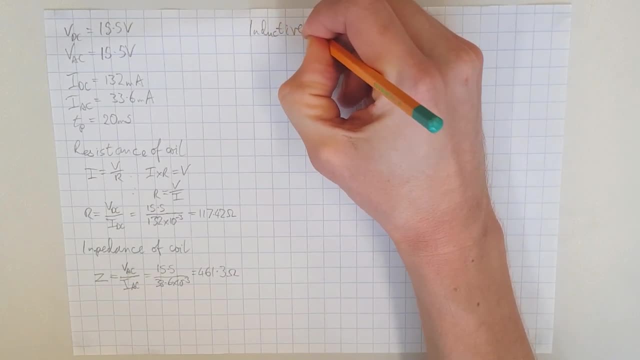 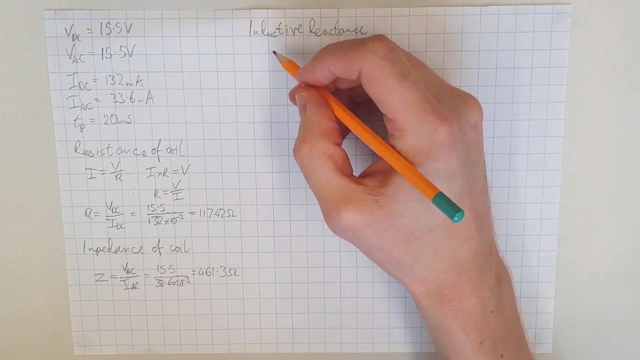 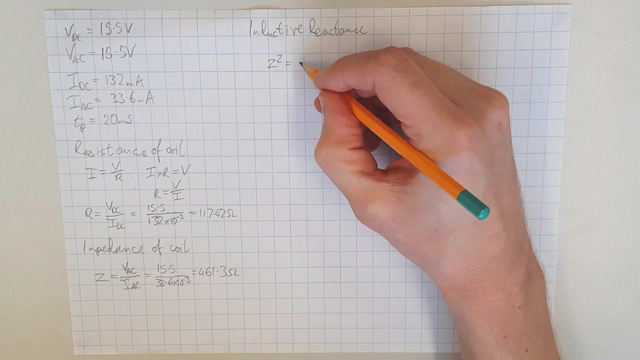 so we're going to try and figure out what is the inductive reactance of the coil. so the inductive reactance and the way that we're going to do that is, we are going to start off by remembering our formula from Pythagoras, which is that the impedance squared in the AC circuit is equal to the resistance squared. 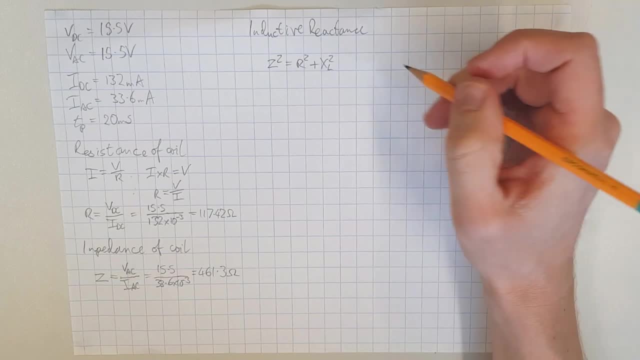 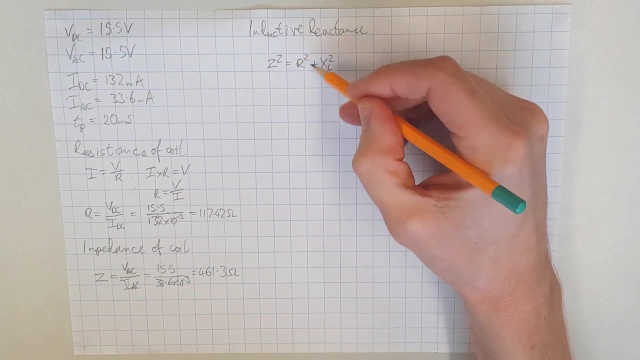 plus the inductive reactance squared. now we're not interested in finding z squared, we're interested in finding xl squared. so what we've got to do is get rid of this r squared first of all. now, at the minute, we are adding r squared, not because of this plus symbol, but because there's a 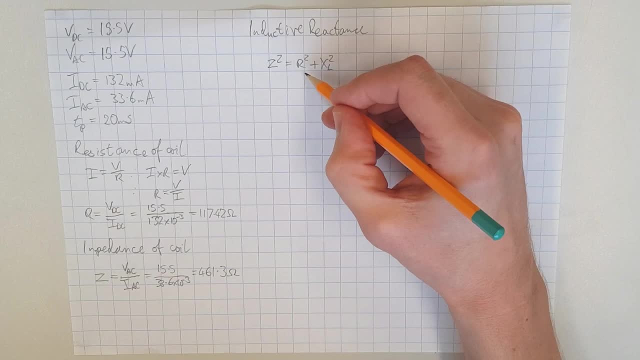 little missing plus symbol here, one of our little ghost symbols. so the opposite of adding r squared is to subtract r squared. and now, just this week, we've got a little ghost symbol here and we're going to continue: além, conspir, MIDY. does it matter which side? the subject goes on? and the answer is: 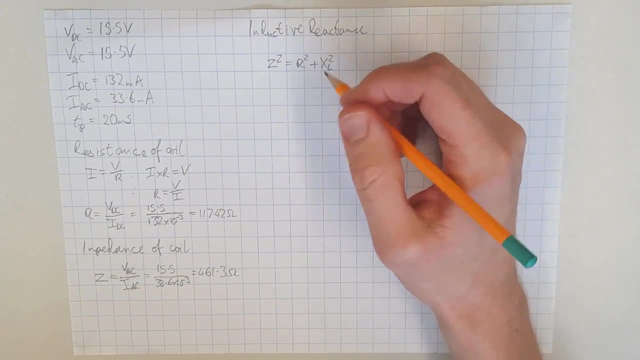 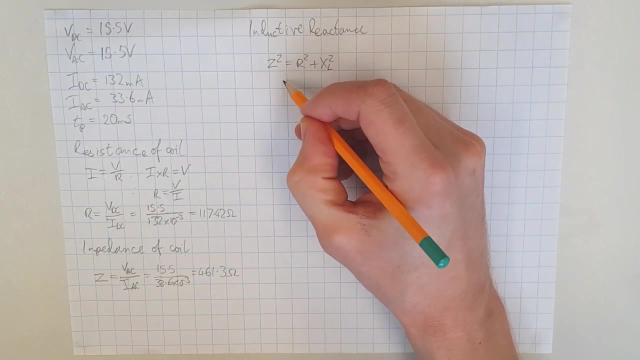 is mathematically no, it makes no difference to the answer, but it's quite nice, from a kind of convention point of view, to have the subject on the left-hand side. so let's just transpose the formula. so we end up with z squared minus r squared from both sides, and if we subtract, 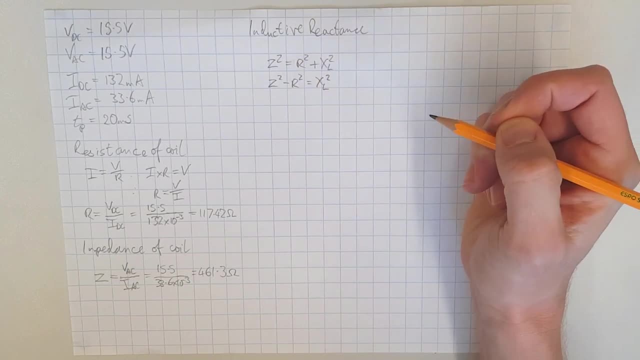 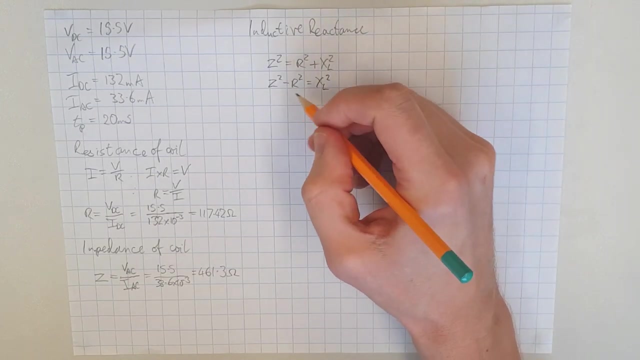 r squared. from this side, we're just left with xl squared. and then, of course, we're not interested in finding xl squared. we're interested in finding xl 2xXL2xL2, or we're interested in finding xl squared, xl by itself. So what we need to do is the opposite of squaring, which is square. 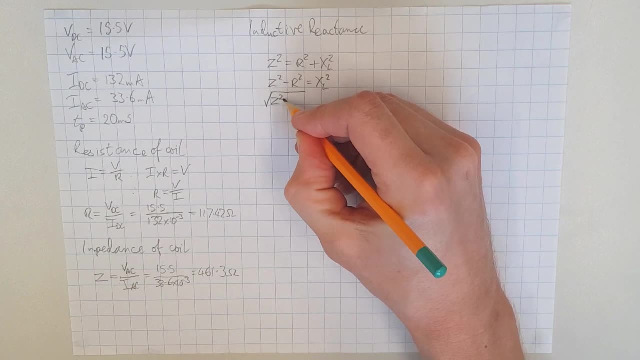 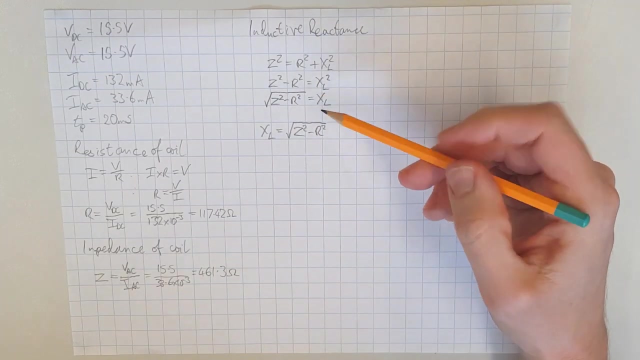 rooting. So we are going to say that is equal to z squared minus r squared, and then square rooted is the same as xl. So we'll just put that down here: by itself, xl equals the square root of z squared minus r squared And, as you can see there, 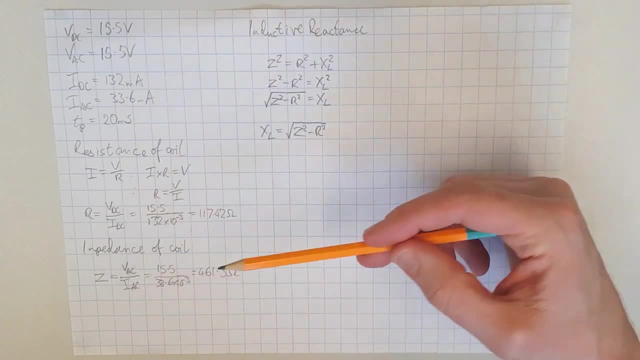 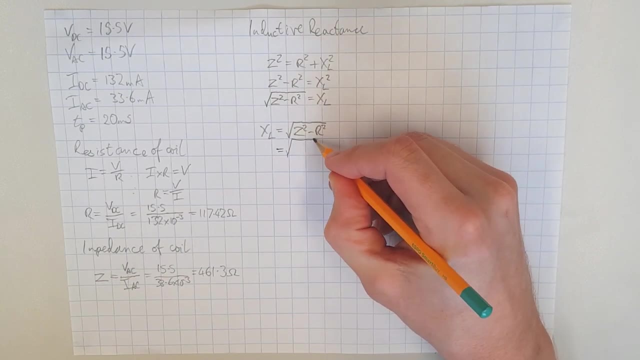 we've got our formula ready to go, So now all we've got to do is put in the numbers that we've already found. So we'll say that xl is equal to the square root of. I've got some numbers to put in here, so we've got the square root of 461.3 squared. 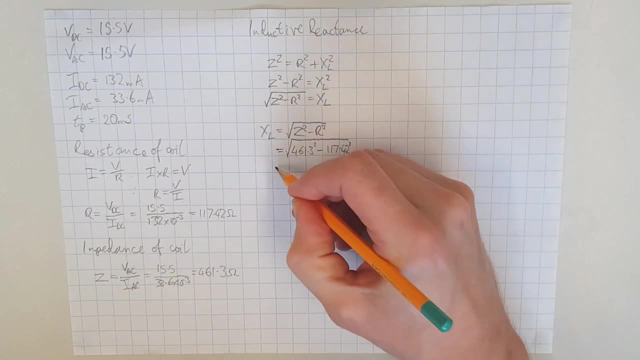 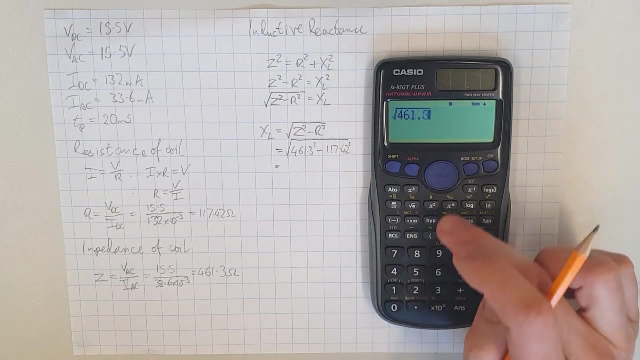 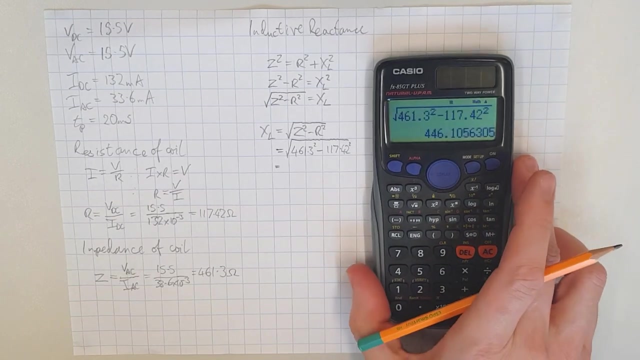 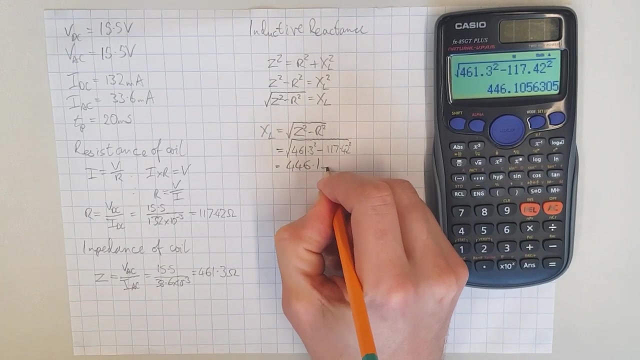 minus 117.42 squared. So let's put that into the calculator and see what our inductive reactance is. The square root of 461.3 squared- take away 117.42 squared- is equal to xl. xl is equal to 446.1 ohms. So the reactive part of that coil offers an opposition to. 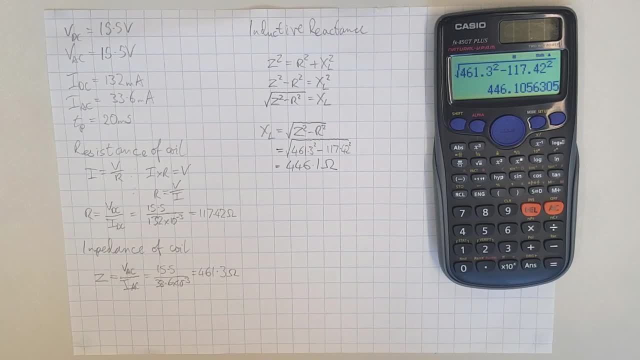 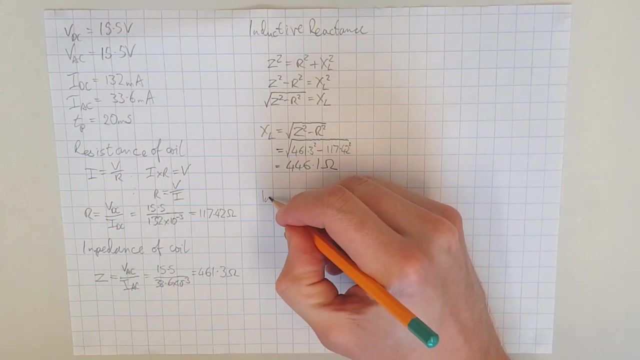 current flow equal to 446.1 ohms. So we've got that value in place now, and now we can use that to figure out some more information about our coil. So the next thing we can figure out is the inductance of the coil. 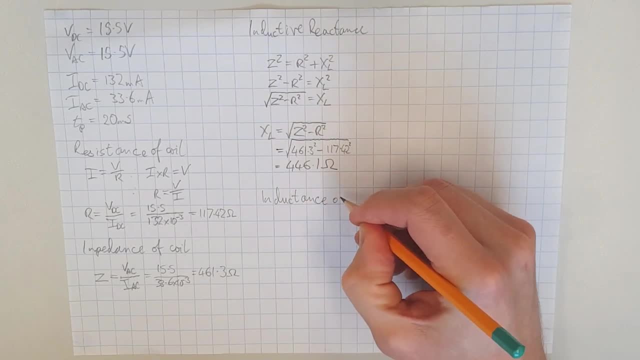 So now we can find the inductance of the coil. Remember, this is just the quality of how good a coil is at inducing a current, either back in itself or into another coil. So we will hopefully remember from previous videos in this series that the inductive reactance of a coil 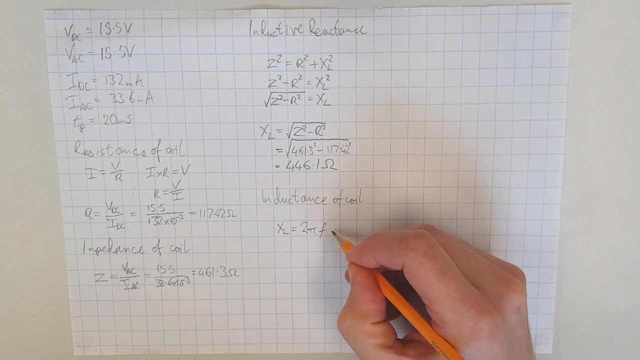 is equal to 2 times pi, times the frequency of the circuit times by l, So l being the inductance of the coil. Now, before we go through this part, I'm going to go through the inductance of the coil. 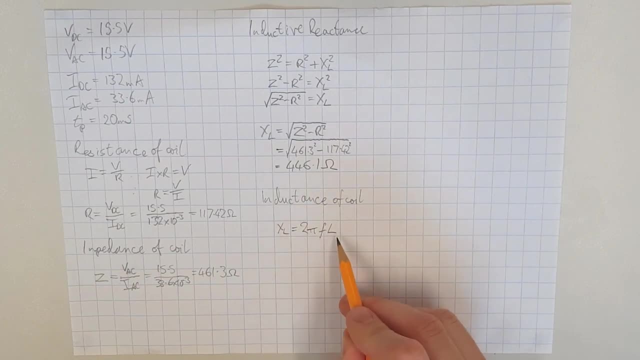 That's the first part of transposing this formula. What we need to think about is: do we have all the information here? Well, we've got xl, So that's great. 2 pi will always be the same. That's a mathematical constant. Do we know the frequency of this circuit? Well, no, we don't. Do we know the? 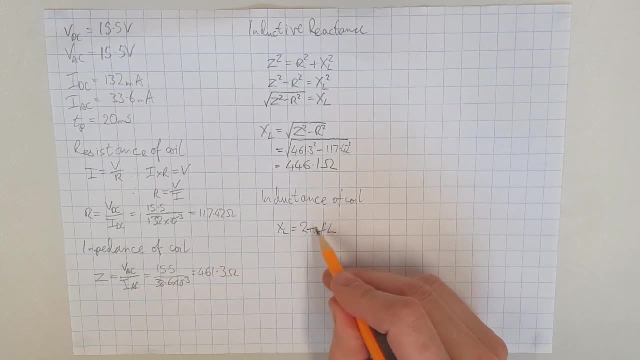 inductance of the coil. That's what we're trying to find, So we're missing this piece of information. But if you remember, from the start of the video we said that the periodic time of the circuit of the AC supply was 20 milliseconds. 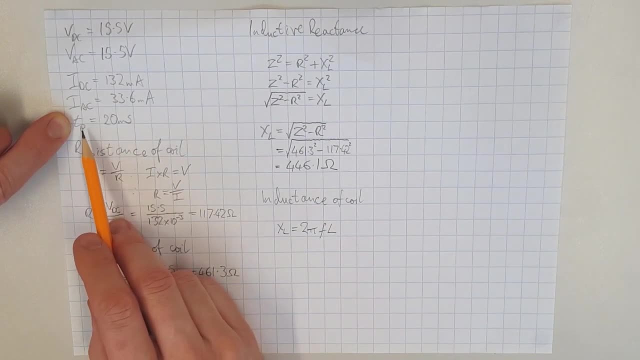 frequency is how many times a complete cycle is completed in the space of one second. So what that means is we basically need to know how many of these cycles are there in the space of one second. If it takes 20 milliseconds to do one cycle, which is what the periodic time is, how many of these are there in one? 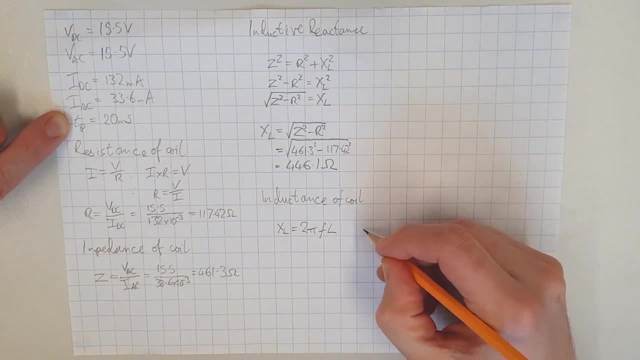 second. So that leads us to quite a nice neat situation where we can say that the frequency of an AC supply is equal to 1, effectively one second divided by whatever the periodic time is. So we can put that in here: 1 divided by 20, now bear. 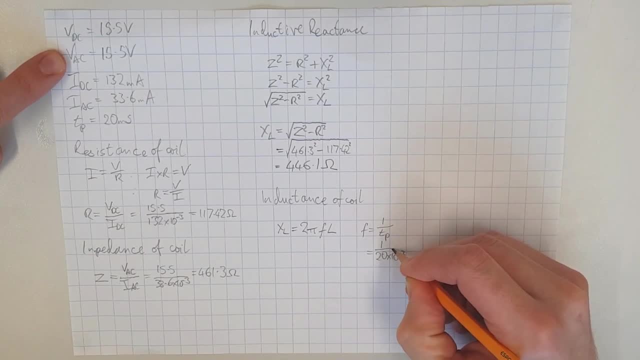 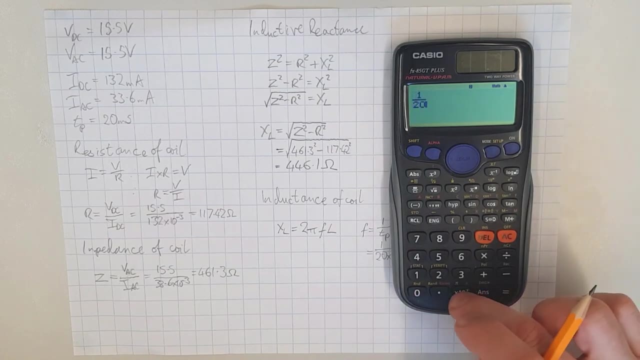 in mind. it's milliseconds, so we're going to do times 10 to the minus 3, which is the same as dividing by 1,000.. So we put that into our calculator now: 1 over 20 times 10 to the minus 3.. And we are going to come out there with 50, which makes 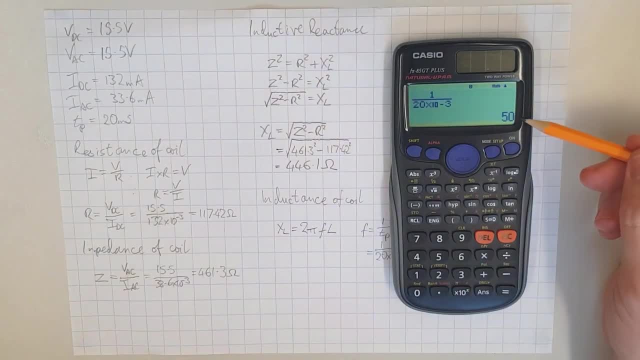 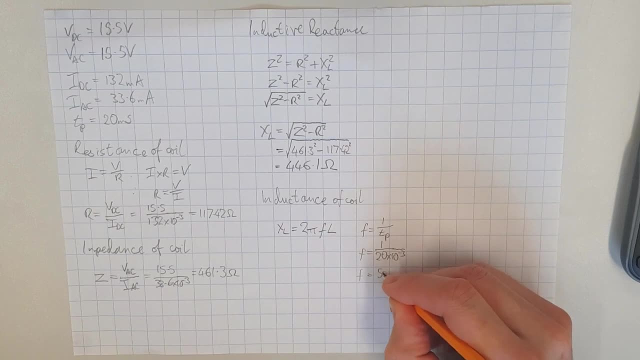 sense, Because we had this connected into a plug socket and we know that in the UK we operate on a frequency of 50 hertz, So the frequency of this circuit is equal to 50 hertz. So now we've got the value we can put in here. So we know this. we know this. 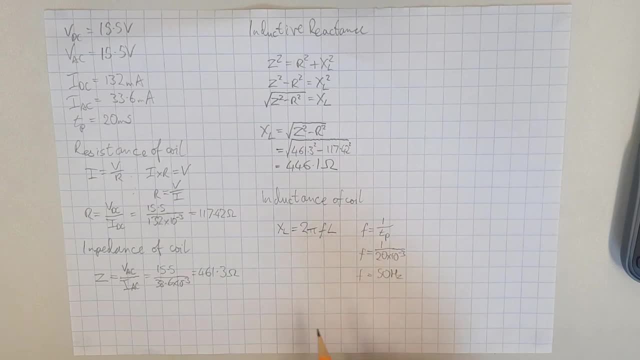 we know this, we don't know this, so we're going to transpose the formula to make L the subject. Now, people sometimes get a little bit confused when they're doing more than one transposition within a formula. The easy way to look at this is: look at L. that's what we're trying to find. And now 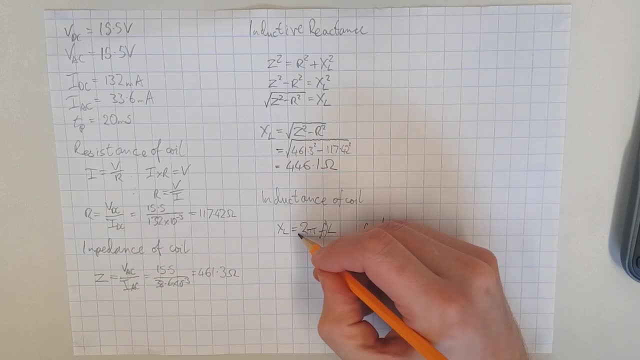 then what are we doing to L? Well, we're multiplying L by this whole chunk here, Just by everything that we've got right there. So then we just ask ourselves: well, what's the opposite of timesing by that big chunk? Well, surely it's to divide by that big chunk. 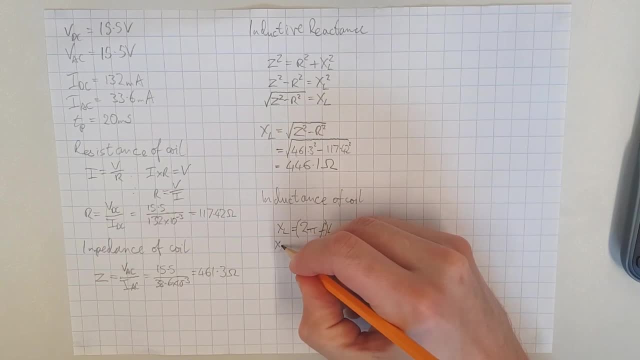 whatever is in there. So that leads us to the conclusion that we divide both sides by that big chunk 2 pi f, and if we divide this side by that big chunk, it just vanishes and we're left with L by itself. So again, let's put L into the. 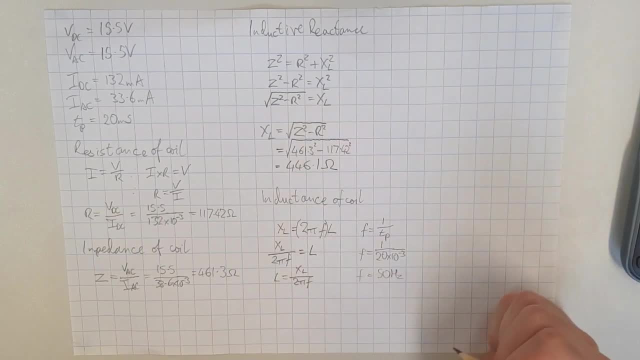 subject on the left hand side, just because that's how most people are comfortable with formulas finishing up, and we're going to volley into here now our values. So we found XL earlier, 446.1, and we're dividing that by 2 pi f, which is 2 times pi times 50. So we'll put that into our calculator. 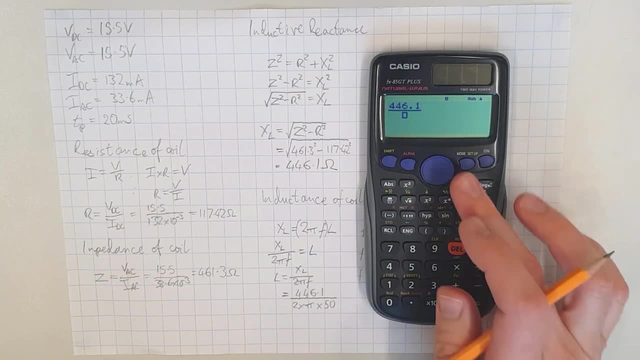 446.1 divided by 2 times pi times 50, and what do we come out with? We come out with 1.42 Henry's effectively. so we've got 446.1 divided by 2 times pi times 50. So therefore, 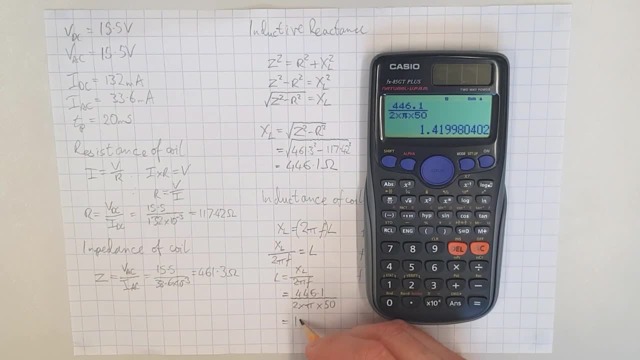 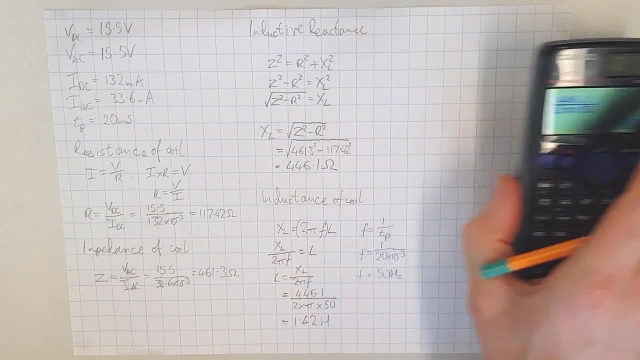 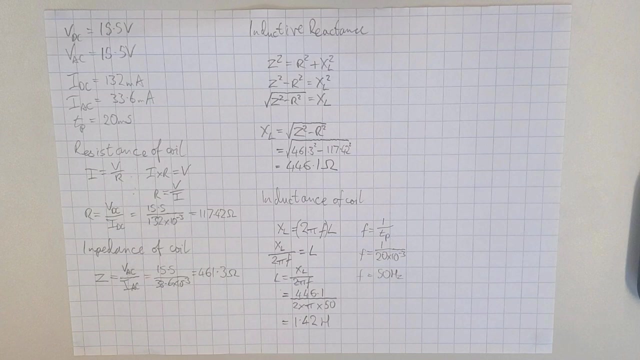 the answer to this part of the question is 1.42 Henry's. So there we go. So we've found out that the inductance of the coil is 1.42 Henry's. So we've already discovered a lot of information about our coil and in the following video we're going to look at information regarding 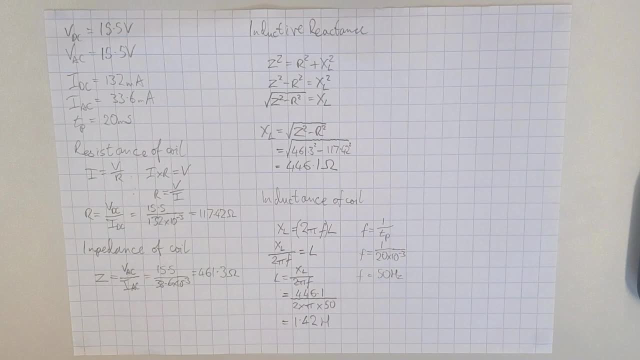 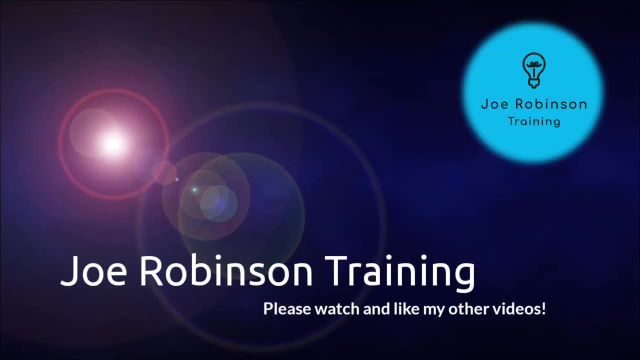 power factor, phase angles and power factor correction. Thank you very much for watching. We'll see you in the next video.